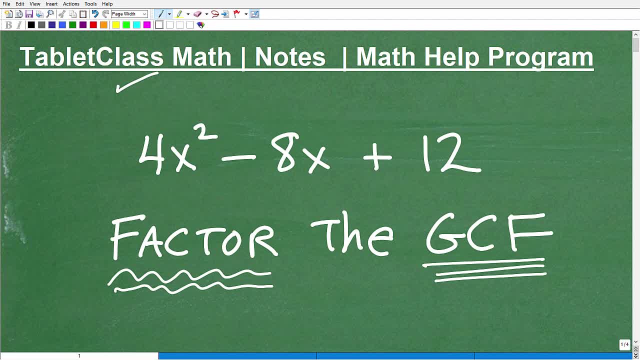 school math teacher And over many years I've constructed a ton of super comprehensive full video-based math courses. So if you need to take an online math class or you just need math help with the course you're taking, I'm going to leave a link to my math help program in the description. 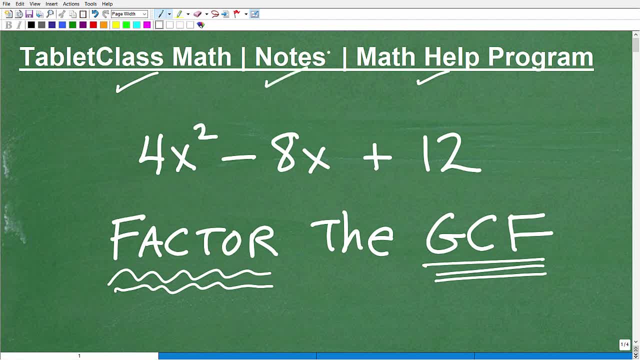 of this video. You can check that out. Also, I offer some very comprehensive notes: pre-algebra: algebra 1, geometry. algebra 2. trigonometry. So if you you know your note taking is not going so good, you need to improve. 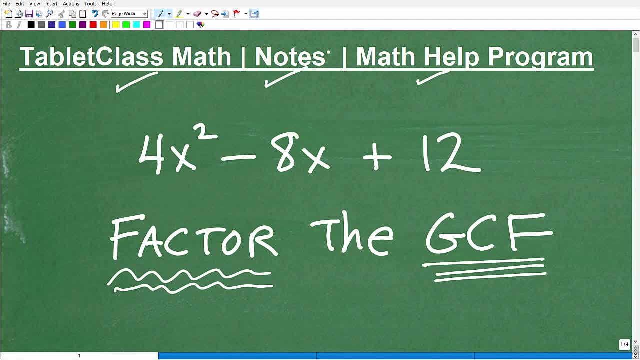 your note taking. Actually, I have some other videos on my YouTube channels on that, But if you're struggling with that, you need a good pair, really good pair of notes. You can find those in the description or underneath this video as well. Okay, so let's get to the greatest common factor. 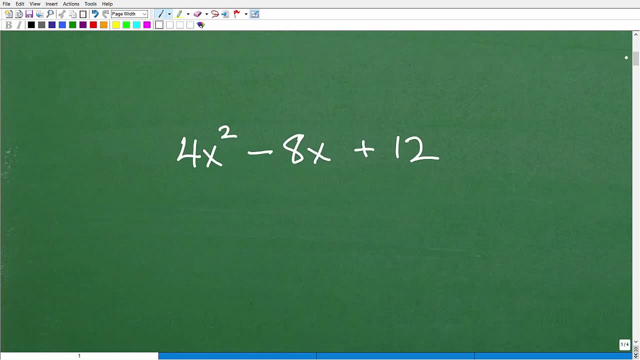 And here is our problem. Now, first thing, let's just talk about number values. So the greatest common factor, the GCF, applies to both. numbers okay, like 4,, 8, 12 here, and variables Okay. 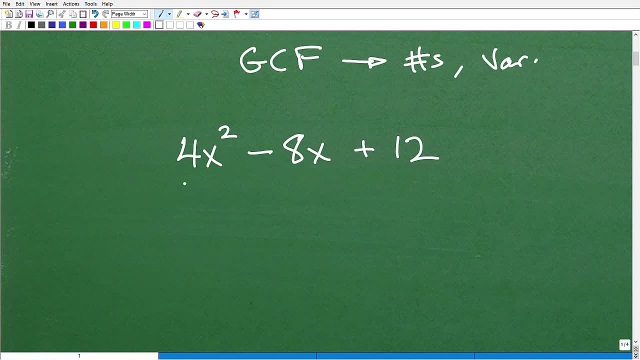 so let's just talk about numbers First off. okay, so we got four. okay, we have this number four, we have this number negative eight, but let's just focus on the eight- And we have 12.. So let's. 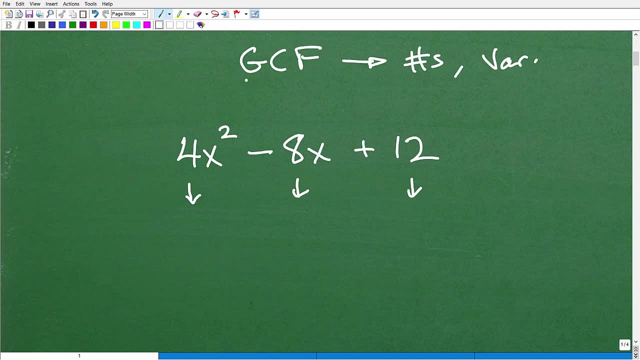 just, you know, revisit the GCF, it's greatest common factor. All right, so let's just talk about factors. So factors are what? Well, factors are ways we can write a number as a product of two or more numbers. So, for example, four, I can write that as four times one. Okay, eight, I can write. 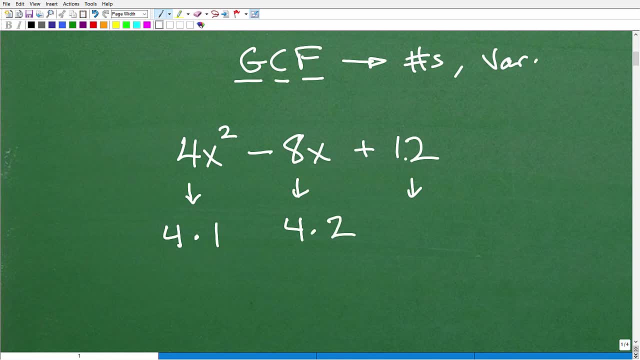 as four times two And 12, I can write as four times three. Okay, Now, that's one way I can write these numbers. Now I can write four. let me kind of just erase this here. So those are one ways. 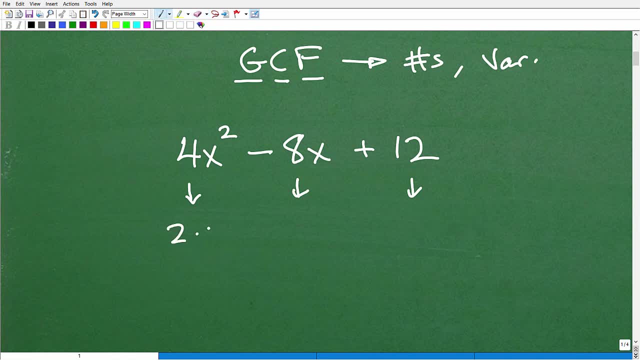 those are factors of those numbers. Now, four, I could also write as two times two. Eight, I can write as two times four. And 12, I can write as two times six. Okay, so let's just talk about each of these values: four, eight and 12.. Now, these are factors. 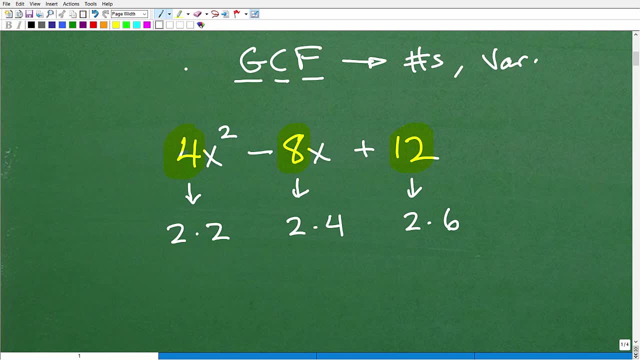 of these numbers. Okay, now we're looking for the greatest common factor. So each of these numbers has factors. right? These are some factors of these respective numbers. So what do they have in common? Let's just start breaking this down. Okay, forget the greatest part right now. What are, what are common factors these numbers? 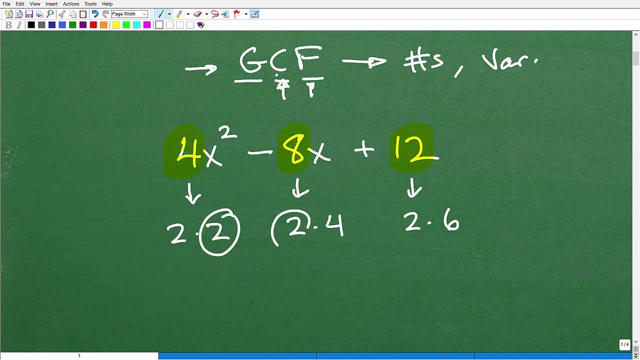 have. So just scanning through it, like, oh, this has a two, this has a two, this has a two. Okay, so do these numbers have a common factor? Yes, they have two as a common factor, So two would be. 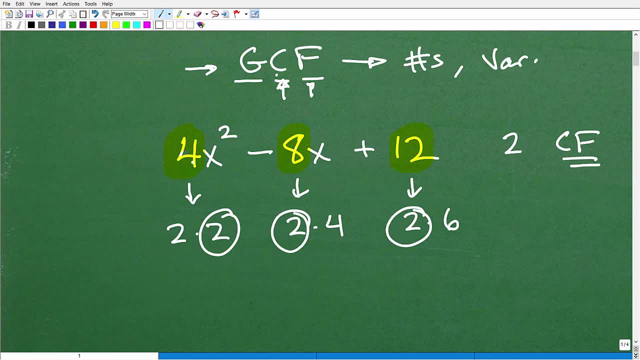 a common factor. okay, for the numbers four, eight and 12.. But I'm trying to find the greatest common factor. I'm trying to find the greatest common factor. So, looking at these numbers, I'm like, yeah, I can write these values differently. I can write again four as four times. 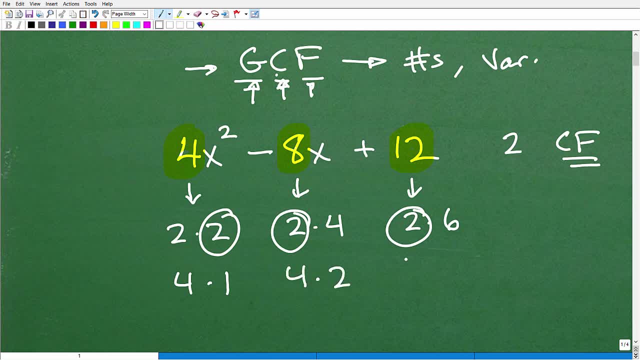 one, eight as four times two and 12 as four times three, that these are also factors of those numbers And I'm like, do I have common factors? Yeah, I have four, And four is the greatest, greatest common factor. Okay, greatest common factor, right. So, although 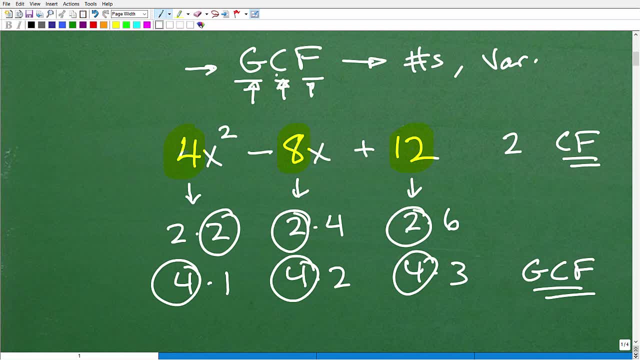 two is a common factor. it's not the greatest. four is the greatest. Okay, All right, So I'm kind of speeding through some things on how we, you know, can break down and find the greatest common factors with more- yeah, more complicated problems, But I just want to try to explain this. 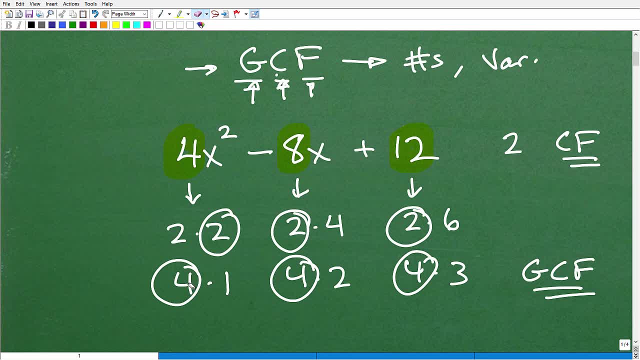 in an easy way to understand. hey, we're looking for the greatest common factor. So you want to be thinking, hey, what's the greatest, the biggest number these guys have in common. So now let's see how we factor this out. All right, so here we have: two was a common factor and four is the. 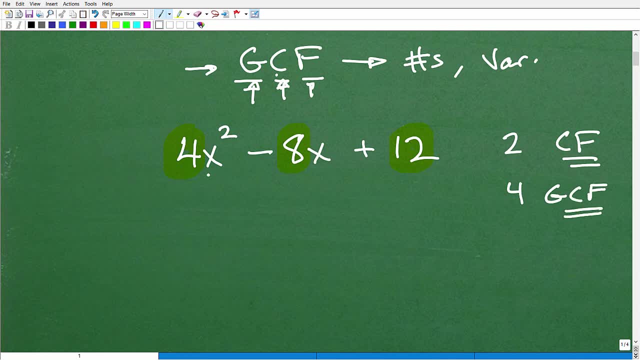 greatest common factor. Okay. So if I was going to factor out a two, the way you're going to do this is you're going to use a distributive property, So you're going to write a two here. Now, this is not. 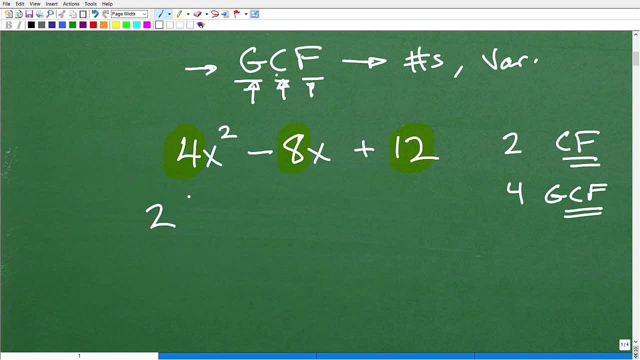 a factor, but I'm just going to show you something. So you're going to write a two here and you're going to put parentheses, Okay, And now you're going to be thinking: let me give myself some more room. You're going to be thinking two times: what gets me back to four x squared? So if you 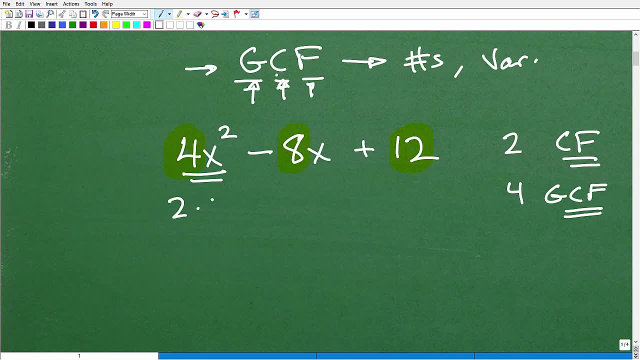 remember. okay, let's just do this here Two times two. This was four times two. or let's do it two times six. Okay, So if I factor out a two to get back to four x squared, I can put a two x squared. 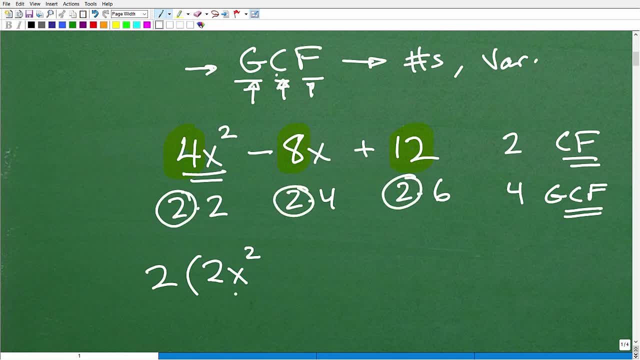 Okay, So I'm taking out a two, So I'm left with a two x squared. Okay, See that, All right. So this is going to be a distributive property situation Minus. what do you think is going to be right here? 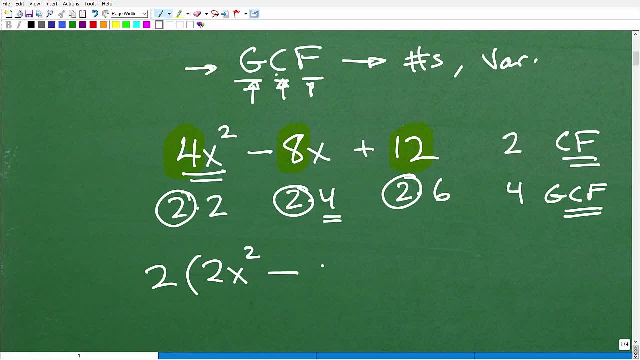 Okay, Well, I'm taking out a two, So I'm left with a four. So that would be four, x, And then what would be plus six? Okay, So here I factored out a common factor of two. I'm left with these values. 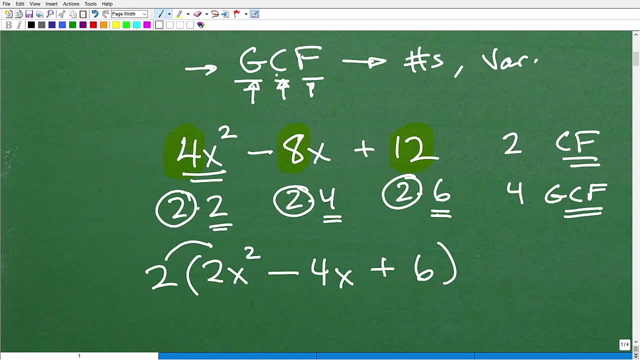 Okay, You kind of see the pattern here, right? That's because if I take this two and I multiply back in using a distributive property, I will get back to the original problem. So I just factored right here, I factored out a two. So what did I do? I factored out a two, Okay. So, but if I look, 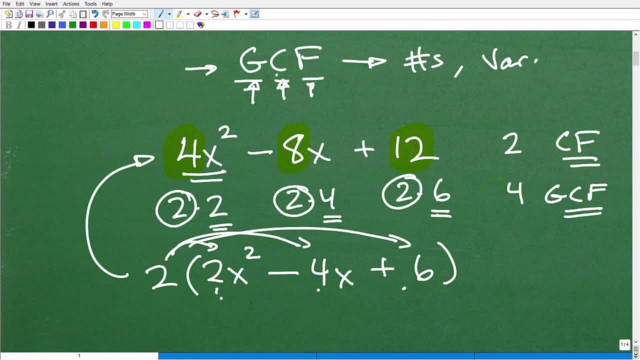 inside. here I'm like man, I can factor out another two. I'm not completely done, So I don't want to do like double work. So let's go ahead and take care of this by factoring out the greatest common factor. All right, So this is the whole idea behind it. So again, remember I had four. 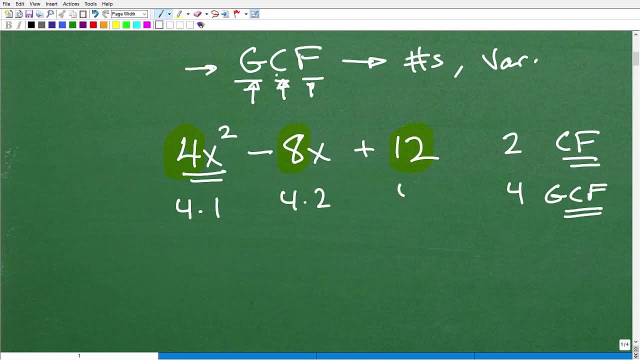 times one, four times two and four times three. This is the greatest common factor, So I'm going to factor out a four. Okay, So I'll write my little four right there. And now, what's left? One. Okay, So that'd be a one X squared, but we could just write X squared. technically Okay, But 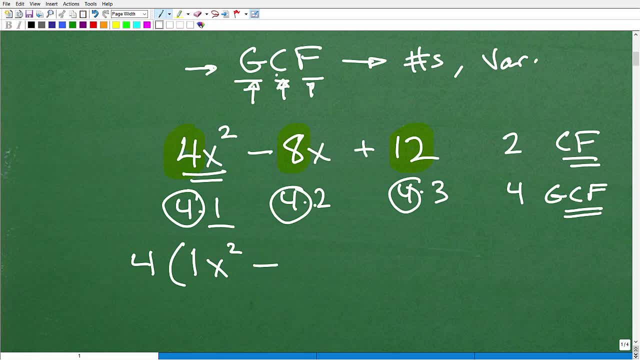 you could just put a little one X squared minus what's going to be left in here. That's going to be two X. All right, Two X plus. you guessed it, That'd be three. Okay, So I just factored out the greatest common factor. greatest common factor right there, Because if I multiply that, 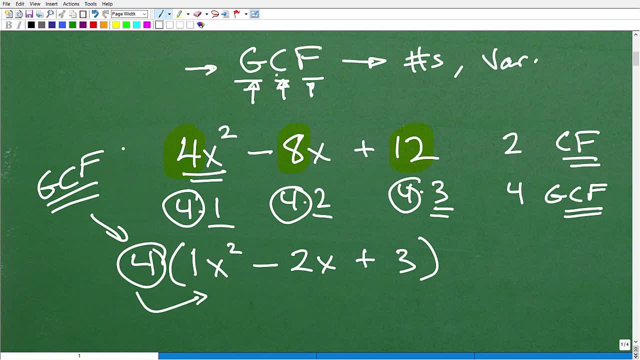 four times one X squared, I get back to four X squared. Okay, Four times negative. two is going to get back to negative. eight X Right, And four times this three is going to get me back to 12.. All right, 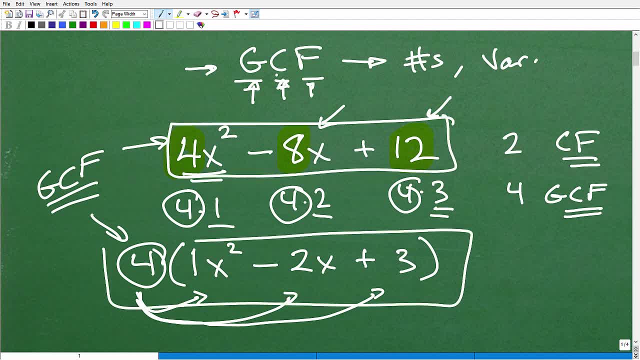 So I took this and I factored out the greatest common factor And that's what you want to do. Okay, You want to factor out expressions, algebraic expressions, completely Okay. So hopefully this is a good quick review, or cleared up. 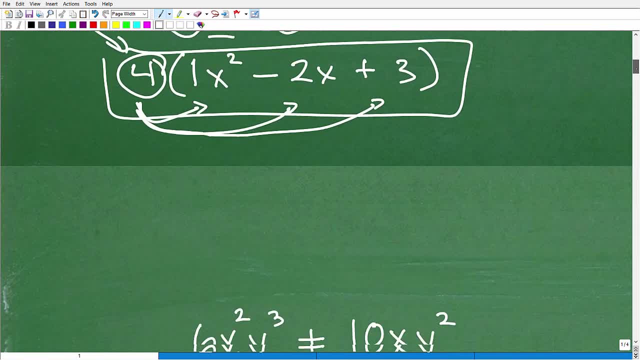 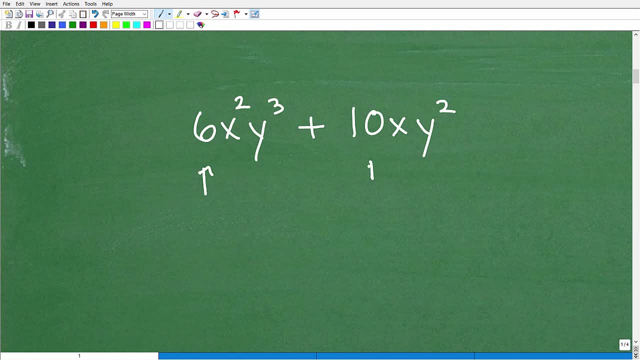 Some confusion. Now let's go ahead and practice this with some additional problems. Now here is a problem that we have both numbers and we have some variables involved, So let's not be afraid of this problem. First of all, let me ask you what is the greatest common factor? Just focusing, 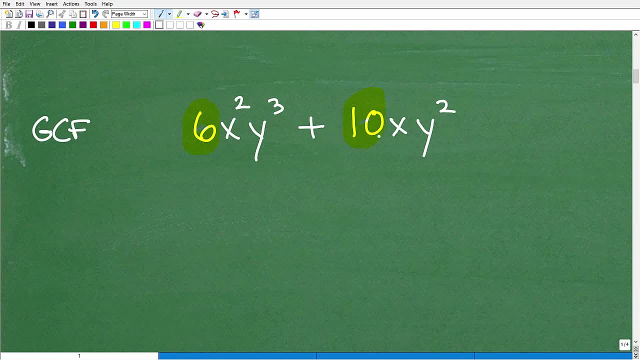 on the number part first. Okay, So when you're doing a problem like this, you're going to have to focus on the number part and then we'll talk about the variable part. So what's the greatest common factor between six and 10?? 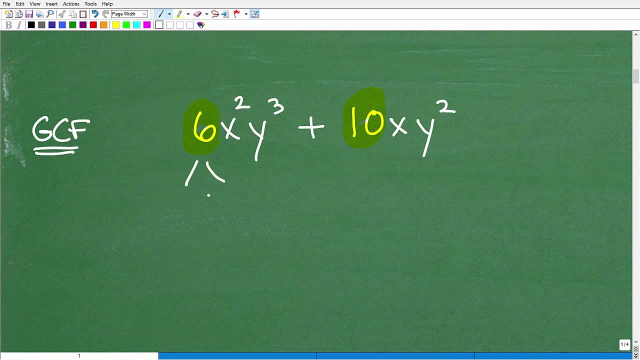 Okay, So let's see about this All right. So we know that this is two times three- There's really not too many ways I can write that Right- And this will be two times five. So the greatest common factor is going to be two. Okay, All right, So two is going to be the greatest common. 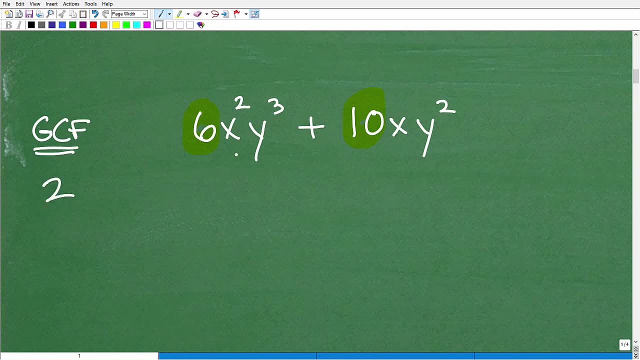 factor. So with the numbers now here we have X's and Y's and the X and Y over here. So the way we factor out the greatest common factor with variables is we have to factor out the greatest common factor. So we have to take, we have to look at what's in common between these terms. 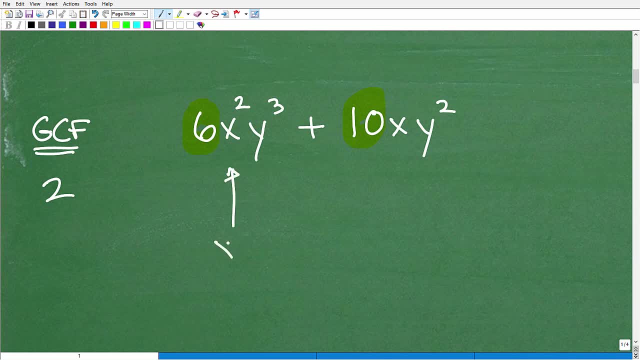 Excuse me, I have an X squared here and X times an X, And then I have an X right here. Okay, X times one. So what is the greatest factor they have in common? This has two X's, but this only. 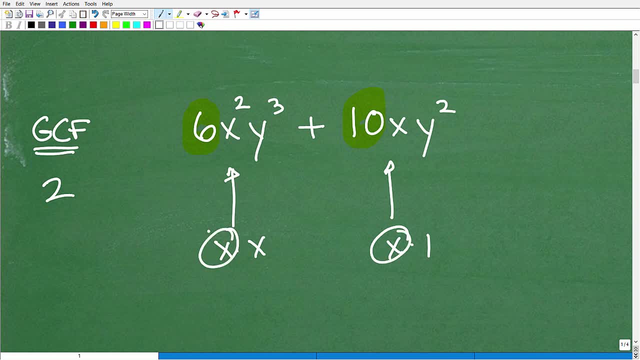 has one, So this has one X here. This also has one X, So one X is going to be part of our greatest common factor. Okay, Not two X's, because they only have one in common. This guy only has one, This has two, but they only have one in common. So how about the Y's? 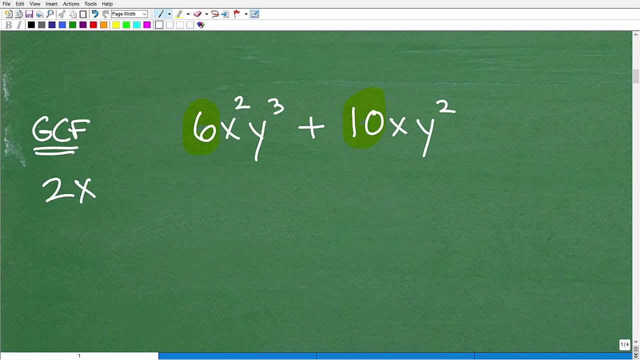 Okay, Let's look at the Y's. So same thing here. This has three Y's, Y times Y times Y, And this has Y times Y, Two Y's. Okay, So how many Y's do they have in common? They have: 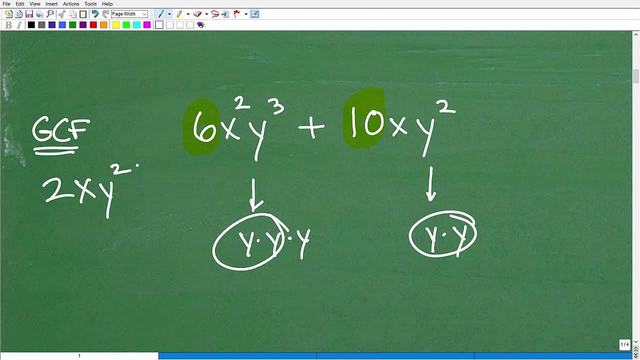 two Y's in common, So that's Y squared. Okay, All right, So that is our greatest common factor. So now, knowing that I can go two X, Y squared parentheses, Okay. Now, what is going to be left in this spot, right here, Okay. 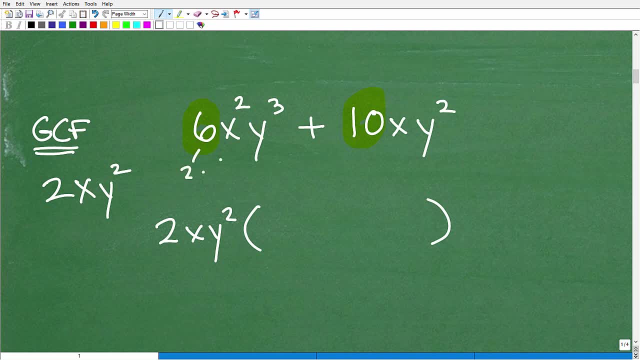 Now, if we just remember when we did our factors, six was two times three, So we'll have a three left. Okay, Now, when I multiply back in, I need to get to an X squared, but I have an X, So I'm. 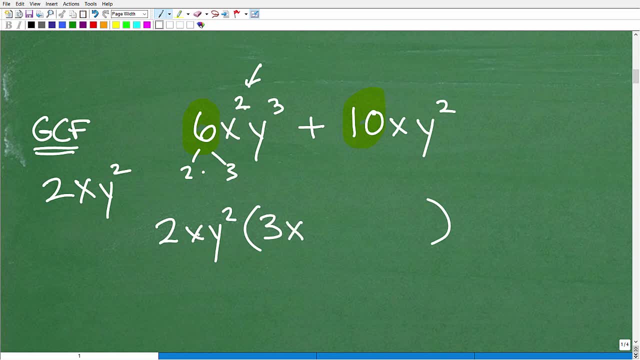 going to need an X there, All right. So X times X gets me back to X squared and I need a Y cubed. So I have a Y squared, So I'm going to need a Y, Okay. So this is going to be my first term plus. 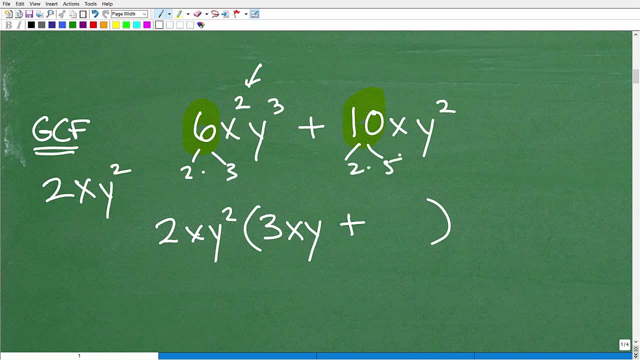 10 is two times five. All right, I have my two, So this is going to be a five, All right, Let me kind of make this a little neater. And to get back to X, Y squared, I already have an X, I don't need. 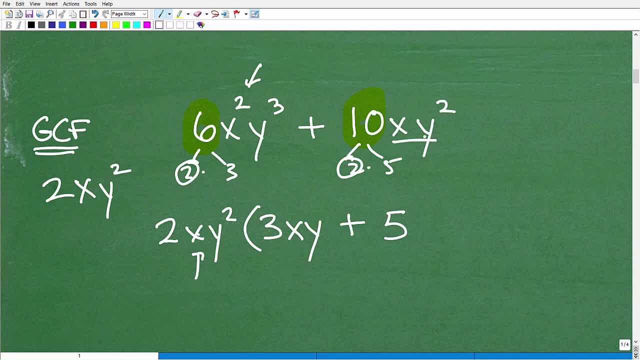 an X, I just, and I don't need a Y squared as well. Right, I have the X and I have the Y squared, So when I multiply back in, I'm going to get back to 10: X, Y squared. So I am done. Okay, So this is. 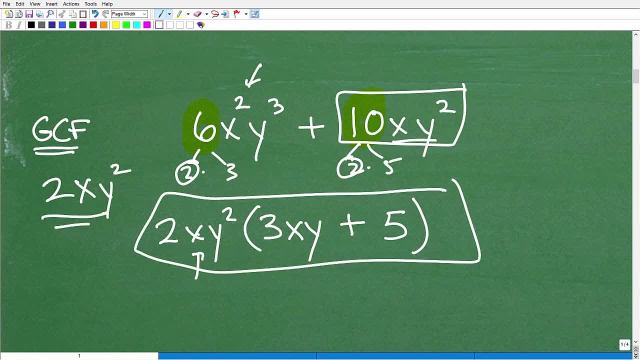 it All right, I factored out the greatest common factor of two X Y squared and I'm left with this. So you can see, uh, to be good at factoring out the greatest common factor, you've got to be good. 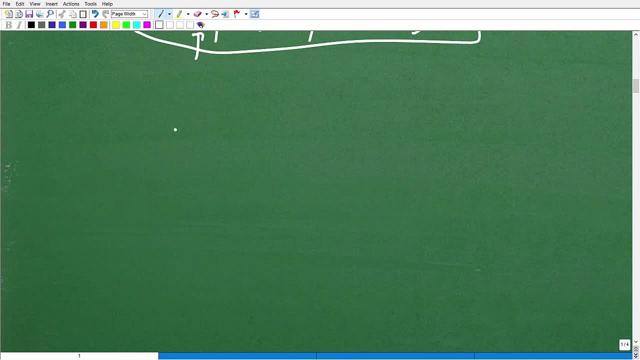 at the distributor property. All right, In other words, you've got to be able to do a problems like three X times four X Y minus two, uh Y, Okay. So, in other words, when you multiply, this is going to be what that's going to be: 12 X times. 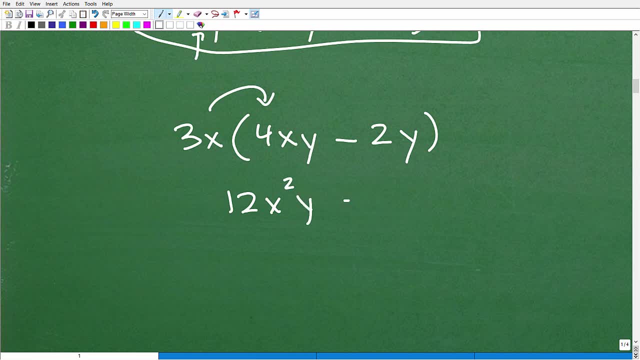 X is X squared, And then we have a Y minus three X times negative two. Y is going to be six X Y. Okay. So if you're struggling with the greatest common factor, make sure you can multiply um using the distributor property. That's another area of weakness for students when they're struggling with the greatest common factor. All right, Let's get back to the distribution property. All right, So let's get back to the distribution property. All right, So let's get back to the distribution property. All right, Let's get back to the. 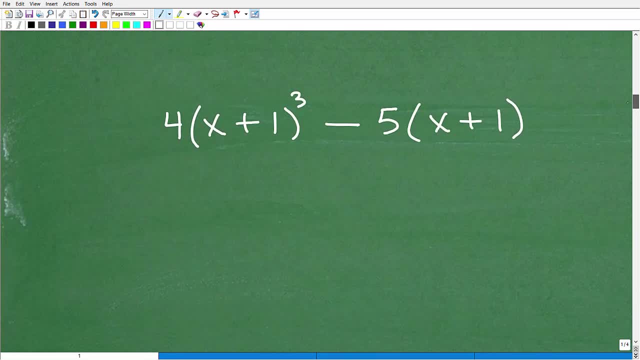 distribution property. All right. So let's take a look at this problem and we'll call this a rep, All right. So how do we factor this out? So if you want to go in and try this real quick and go ahead and do that, Okay. So we're like: okay, I have numbers, but I don't have any like common. 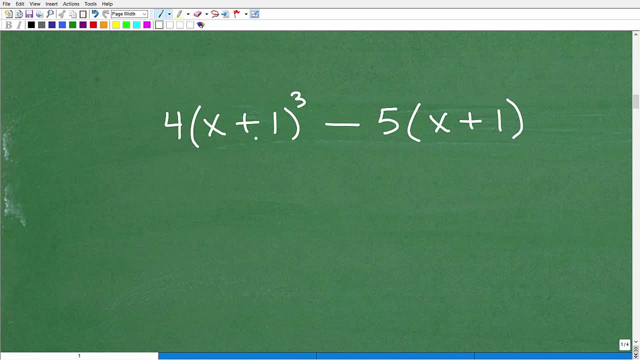 factors between four and five. That's hopefully pretty obvious. but here I have an X one X plus one cube, So this is really X plus one times X plus one times X plus one. Okay, That's what this means. And then I have an X plus one times X plus one times X plus one. Okay, That's what this. 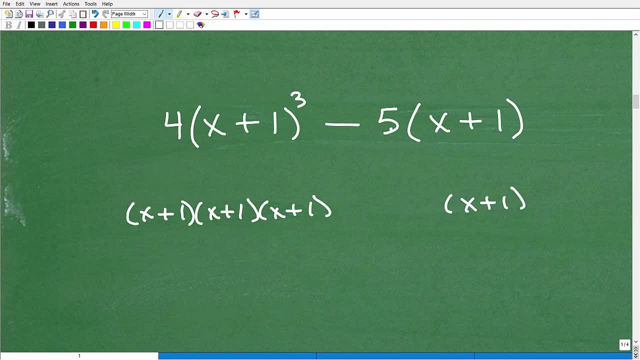 means. And then I have an X plus one times X plus one times X plus one over here. So we do have some common factors, right? These are factors. This is five times that and this is four times this. Okay, So what are some common factors? This is all multiplication. Well, I have one here and 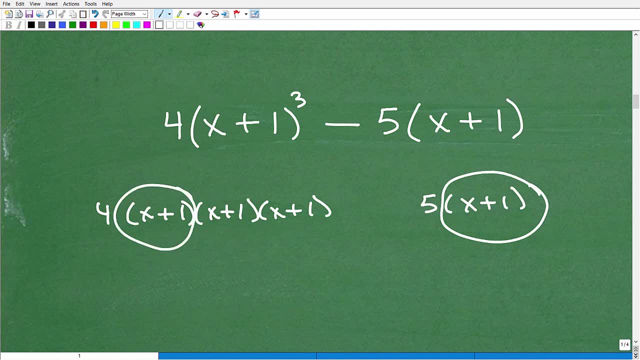 I have one over here, I have three, but I could, uh, I have one in common. So X plus one is my GCF. My GCF is X plus one. Okay, So if I factor out my GCF, let's do it down here. 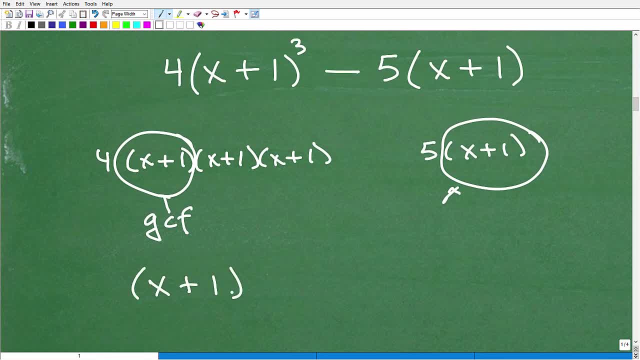 Okay, That's going to be X plus one. All right, What's going to be remaining? Well, my four will be remaining, my X plus one. right here, I have two of them, so I can write that as X plus one, squared minus. uh. and what's left over here? just a five, five, Okay, And there is my answer. 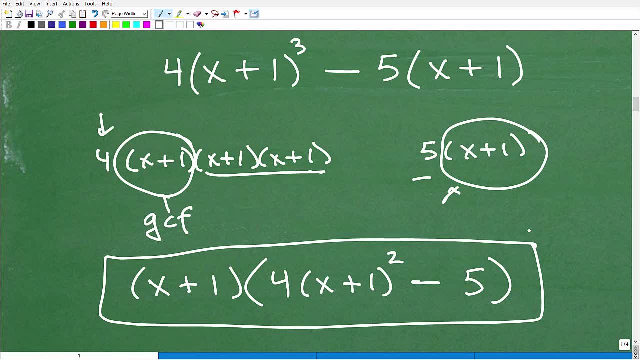 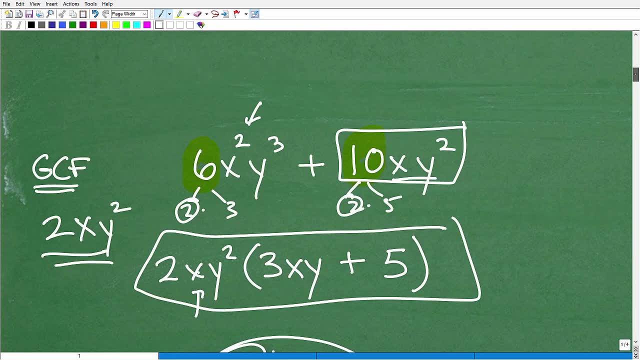 Okay. So greatest common factor Again: start with the basic, easy problems. When you're doing this- whether you're taking a- uh, I'm assuming you're studying this in some sort of math class- go go through and make sure that you do all your easy problems first. Okay, Then work your way up. 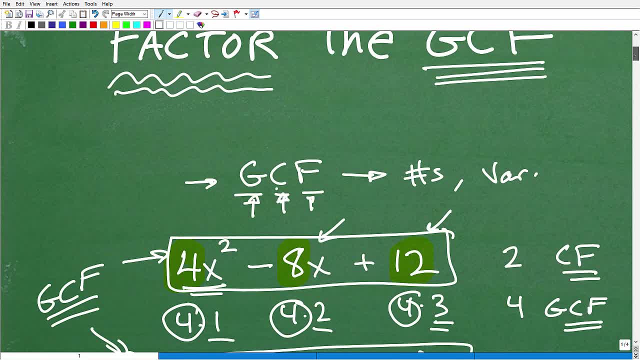 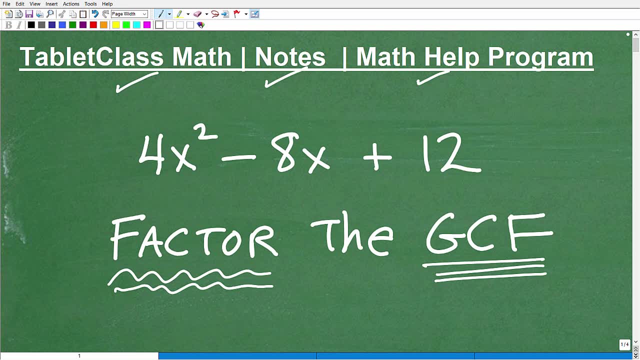 get the concept down. Okay, Uh, I try to cover a decent amount of ground in this video, but hopefully you know, uh, this cleared up some conceptual confusion that you might've had about factors and common factors And, of course, the greatest common factors and how we can kind of 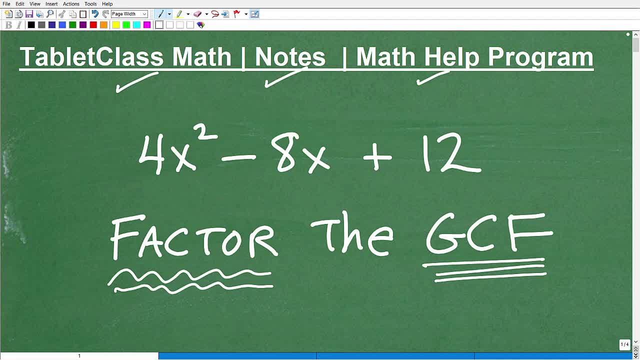 see them in these problems. The bottom line is you need to know how to factor out your factor And, quite frankly, you're not going to master factoring and um you know? quick video like this- or this is this video- is designed to help clear up some confusion. teach you real quick. 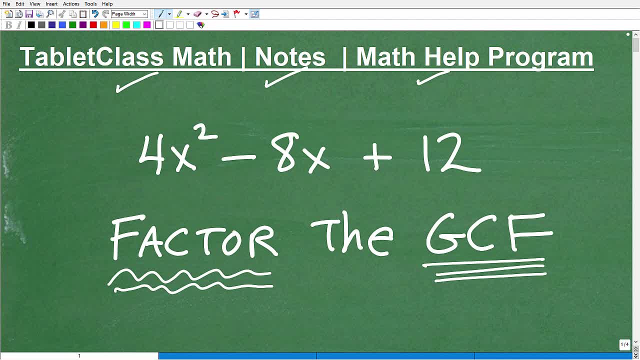 but you know it's really not a complete full lesson And, uh, it's not going to really do you much help unless you practice. You've got to practice, practice, practice. So if you want to see a ton of videos, a ton of problems with video demonstrations, and you'd really need that kind- 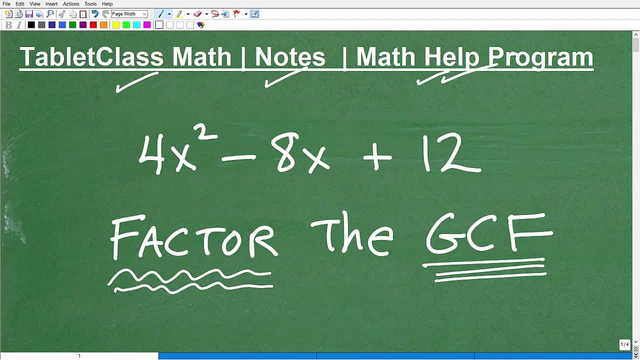 of support, then you would definitely want to check out one of my math courses. I would suggest maybe, like uh, algebra one. Um, I really get into uh factoring pretty heavy duty there, Uh, so of course, any of my other courses above and beyond. 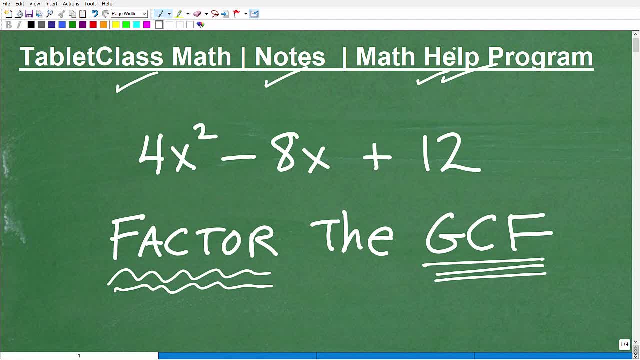 that, uh, I'll have factoring in there, Not so much in pre-algebra- and pre-algebra we kind of get used. Yeah Well, we are talking about the greatest common factor in pre-algebra, but more in a basic sense And of course, um, I know it's going to help you out And I do have other. 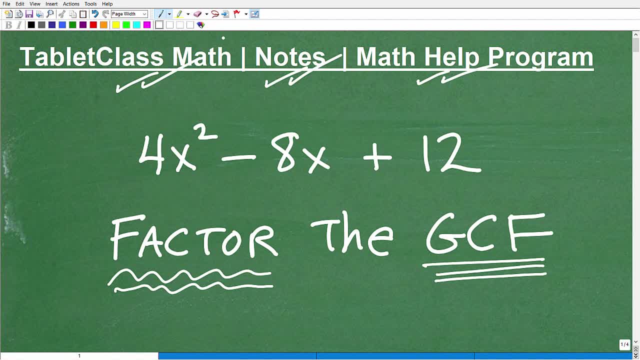 videos on the greatest common factor on my YouTube channel. But if you found some value in this video, I definitely appreciate you smashing that like button And, uh, hopefully, uh, if you like my teaching style, uh, please consider becoming a subscriber. 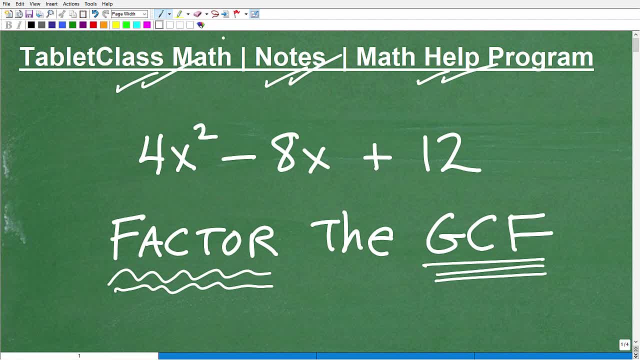 I'm posting stuff all the time. I've been on YouTube for 10 plus years. Uh, as you probably can tell, my passion is teaching math. So if I'm helping you out, then I'm doing my job, Okay, So 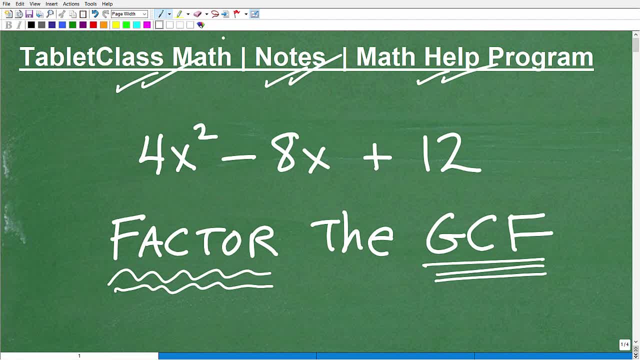 with that being said, I definitely wish you all the best in your mathematics and adventures. Thank you for your time and have a great day. 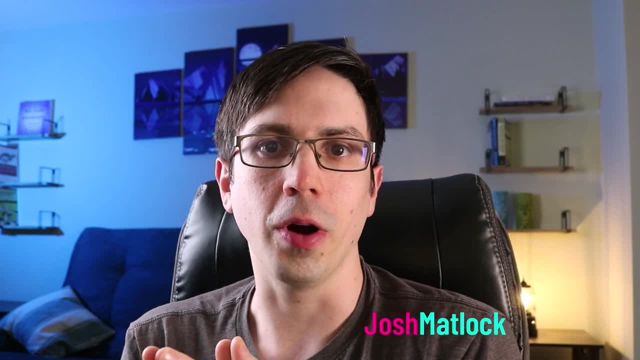 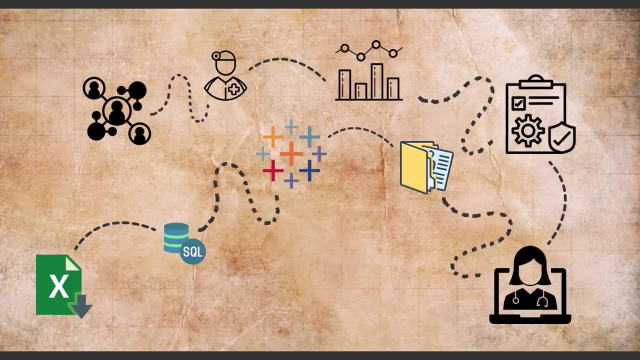 Today I'm going to try and do something that I don't think has been done before. I'm going to try to create a healthcare data analyst roadmap. Now, it's impossible to be an expert in everything in healthcare. There's so many different places that you can work.